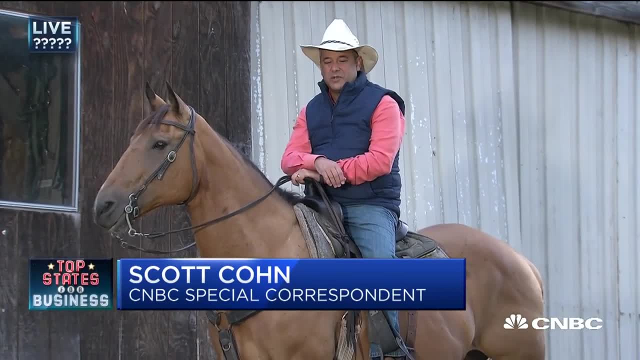 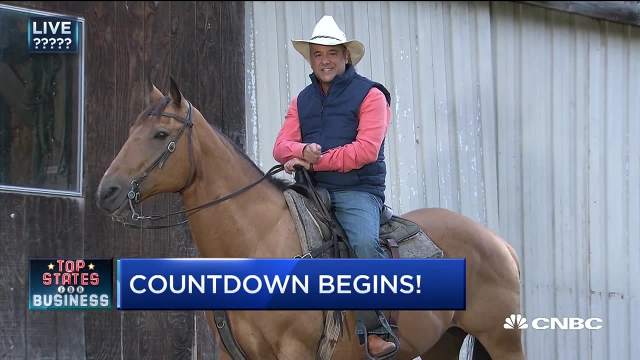 So listen, here's the deal. We're going to count down the top states for business all day today, And this is a study that we've been doing every year for the last 11 years. We rank every state on 66 metrics in 10 categories of competitiveness, for a total of 2,500 points. And what we'll be? 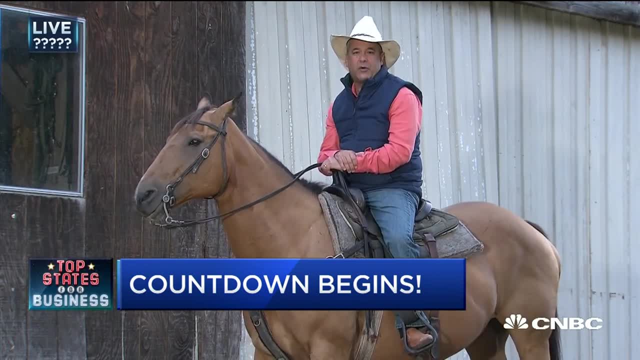 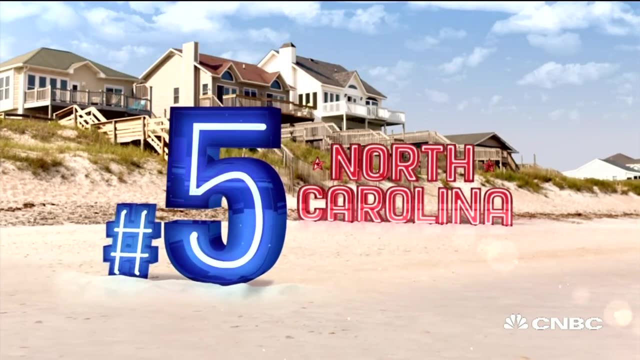 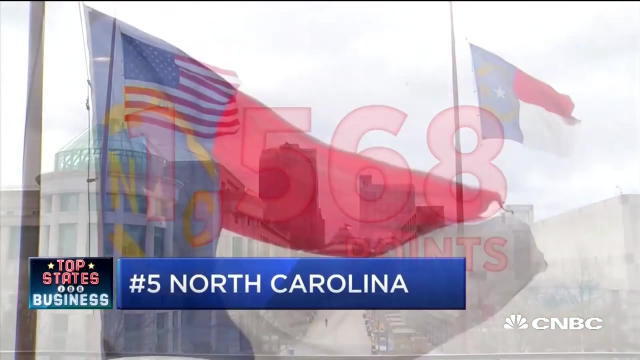 doing today is counting down the cream of the crop. So let's get our countdown going now. Here's state number five, North Carolina. the Tar Heel state comes in at number five this year with 1,568 out of 2,500 points. North Carolina also finished fifth last year. 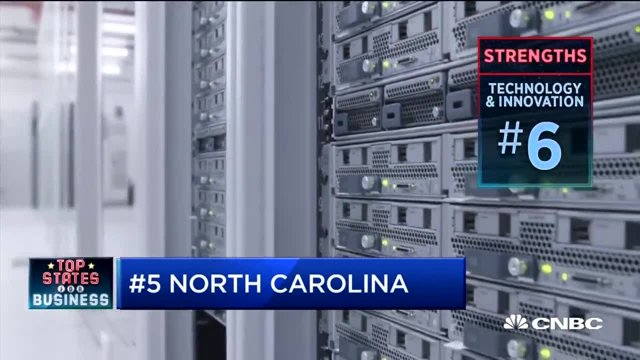 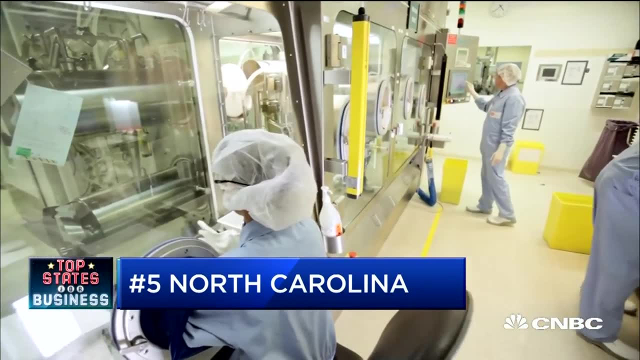 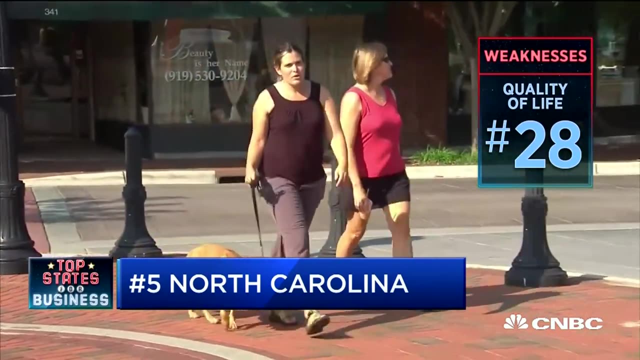 North Carolina's best category is technology and innovation, a perennial magnet for research and development. that also helps the state notch a top 10 finish in the important workforce category. But cuts in school spending dropped the state to 32nd for education and it's 28th for quality of. 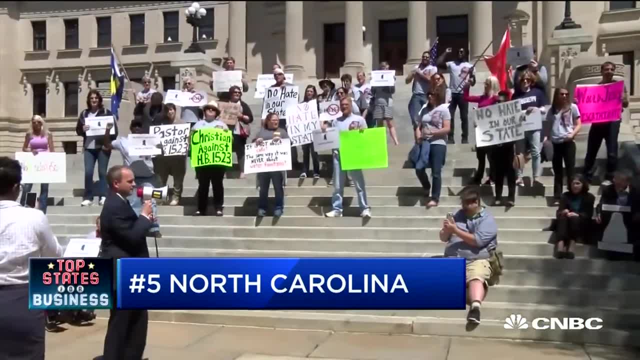 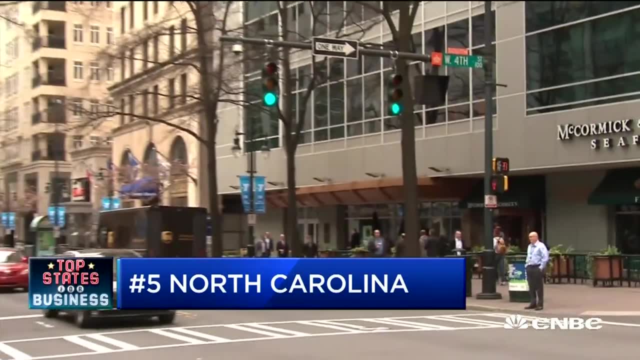 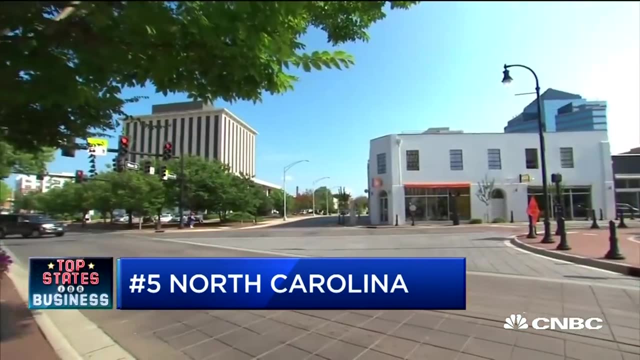 life. North Carolina repealed its controversial ban A bathroom bill, so businesses and events that boycotted the state have begun to return, But it is still one of only five states with no anti-discrimination laws for non-disabled people, making it one of the least inclusive in the nation. 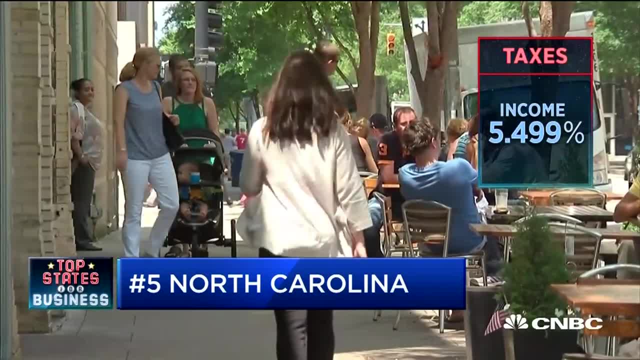 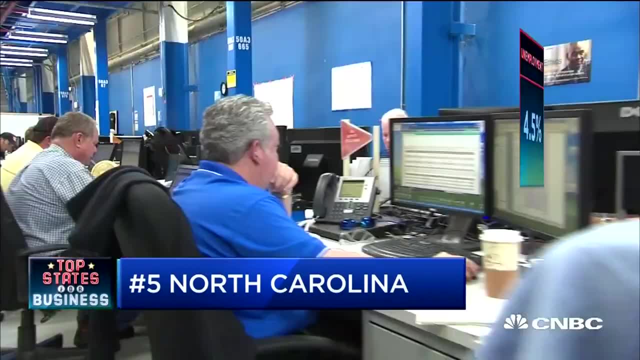 North Carolina's individual income tax rate is a flat 5.499 percent. The corporate tax is 5 percent. The top state sales tax is 7.5 percent. Unemployment is 4.5 percent. North Carolina's largest employer is Walmart. 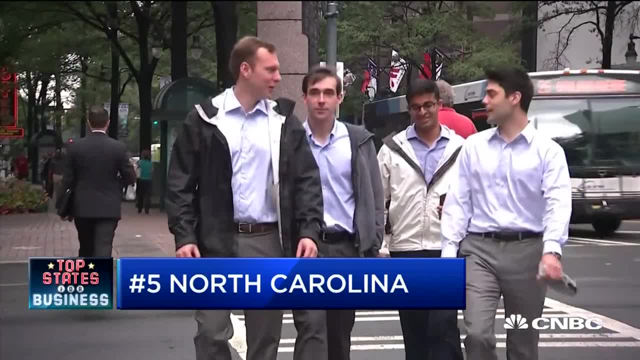 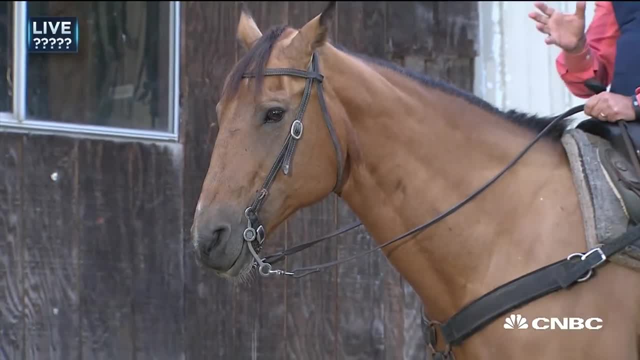 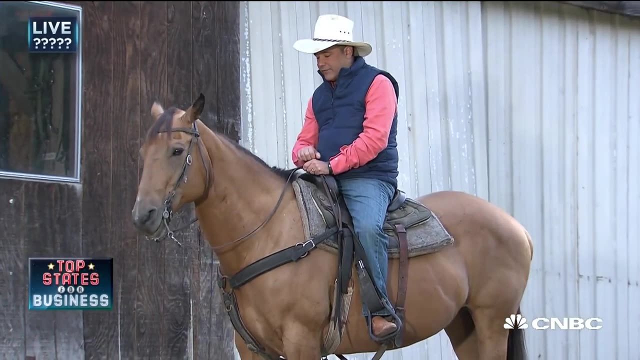 The largest industry is professional and business services. So once again, for the second straight year, North Carolina- were it not for that quality of life ranking or the education ranking- might have been at the top of our list, but it comes in again at number five for a second straight year. 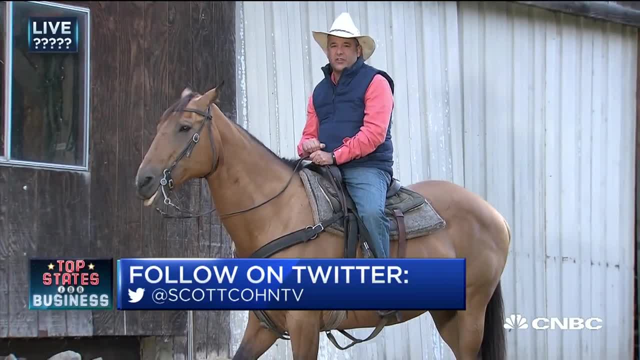 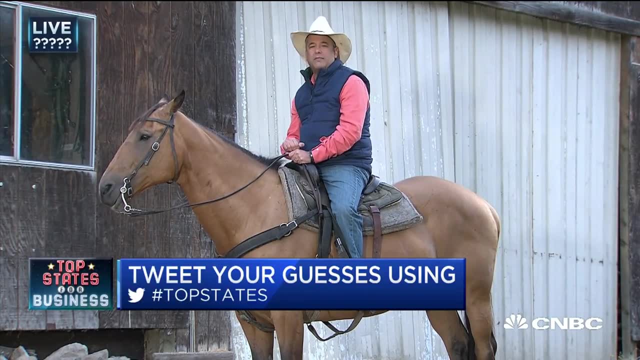 So where am I? America's top state for business? Here's another one of our diabolical hints: You can't get there from here. You can't get there from here. What does that mean? Think about it, Think about it. Try and get into this hat and under this cowboy hat, You like this? 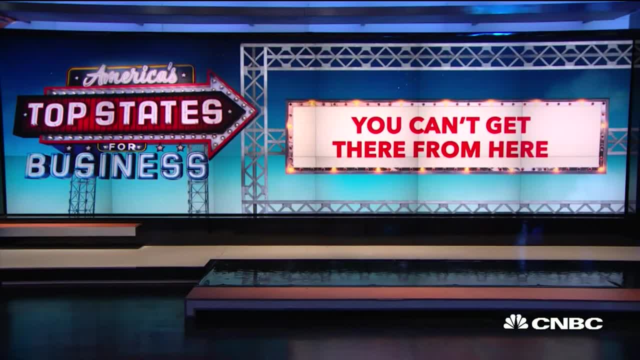 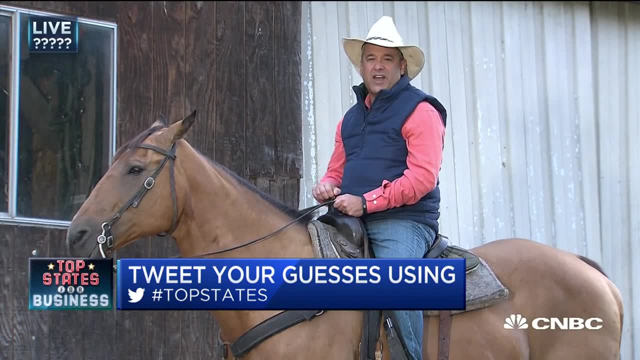 And you can read all about our study: topstatescnbccom. Follow us on Twitter. Use the hashtag topstates. Let us know where you think I am. We'll have another state in our countdown coming up on Squawk on the Street, guys. Thanks for watching.